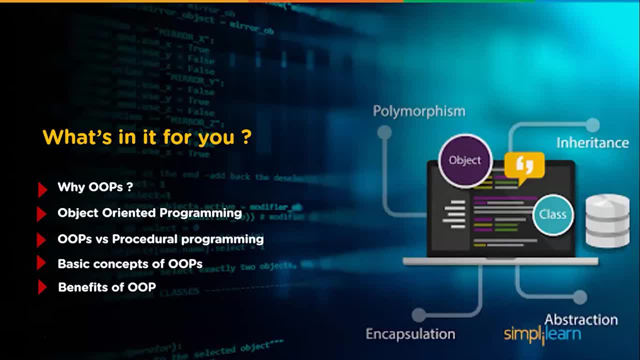 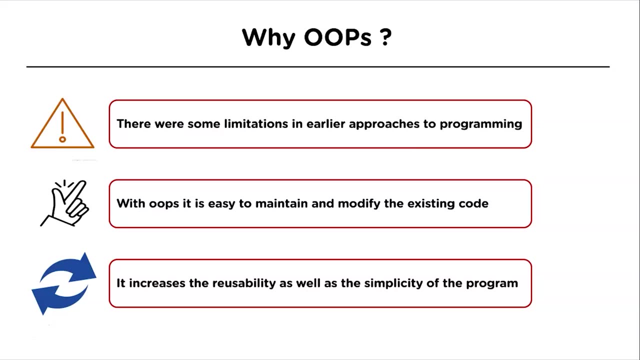 concepts of OOPs and at last, we will learn about the benefits of OOPs. But before moving forward, make sure to subscribe to our channel and hit the bell icon to never miss an update. Now let's move on to our first topic. that is why OOPs. Well, there were some limitations. 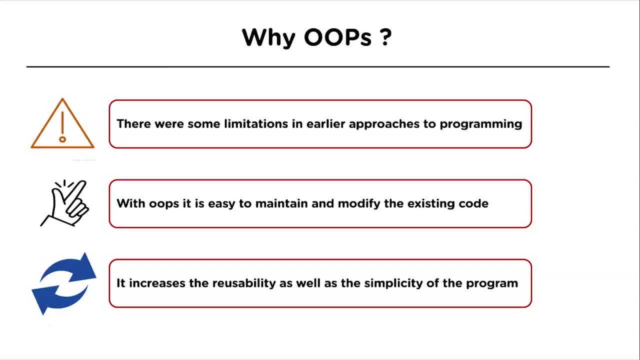 in earlier approaches to programming, and OOPs help to fill those gaps. In object oriented programming, it is easy to maintain the code with the help of classes and objects and with the help of inheritance. there is code reusability, that is, we don't have to write the same code. 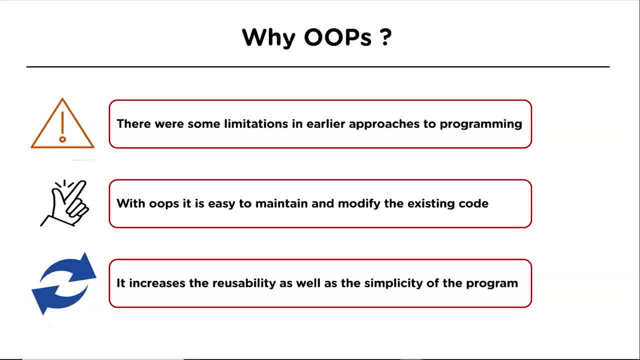 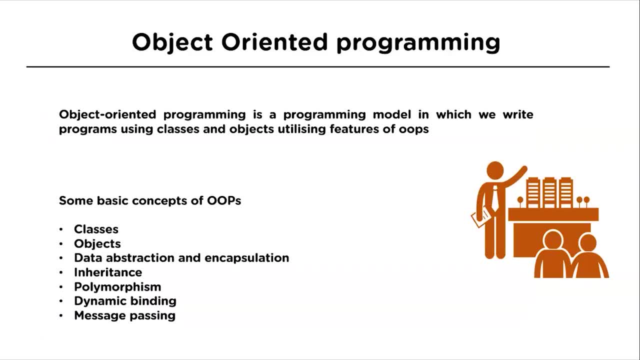 again and again, Which increases the simplicity of the program. Now let's understand what is object oriented programming. Object oriented programming is a programming pattern where the programs are structured around objects rather than logic and functions. In other words, OOPs basically focus on objects that are required to be manipulated instead of logic. For example, let us suppose 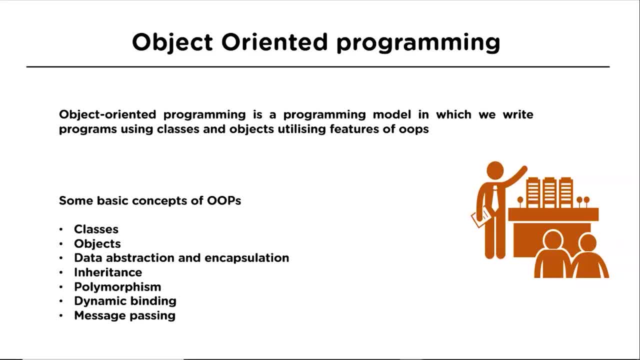 we have made blueprint of a mall, then that blueprint will be a plan that explains what it should look like, etc. But it is just a blueprint of the mall. we cannot go inside it physically as of now. Now the constructors will go through the blueprint and they will 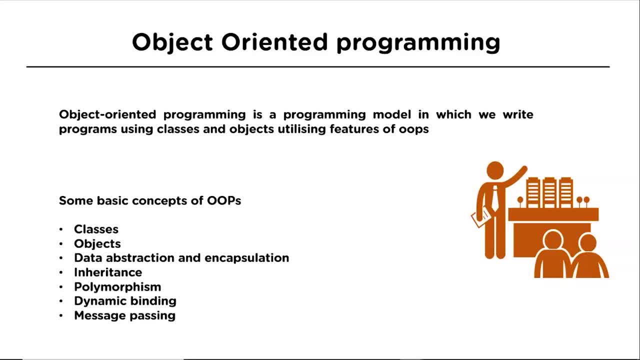 construct the mall and they can make as many malls as they want with the help of that blueprint, and each mall can have its own different shops and showrooms. In this case, blueprint is the class, the mall is the object and the shops and showrooms inside the malls are the 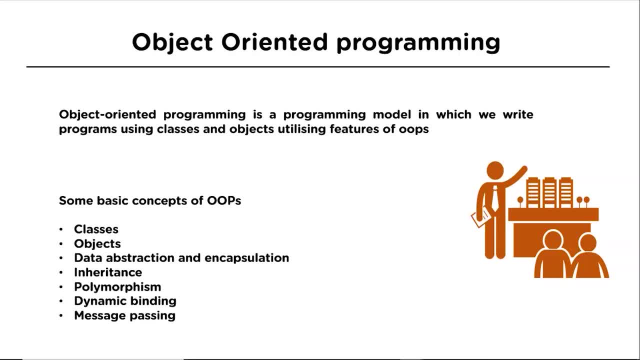 data stored in the object's properties. And these are some basic concepts of OOPs. First is classes, then objects, then data abstraction and encapsulation, then there is inheritance, polymorphism, dynamic binding and message passing. We will learn about these. 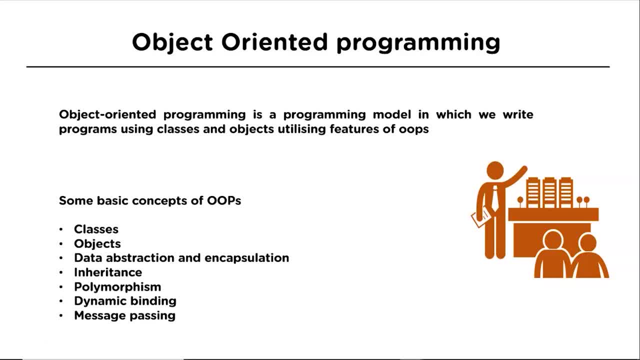 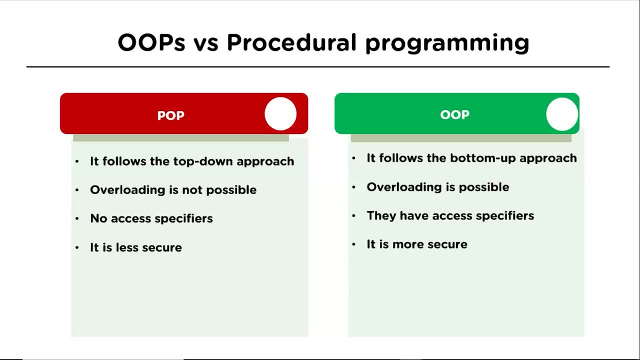 concepts later. First, we will discuss the difference between OOPs vs procedural programming. Procedural programming follows top-down approach Here. top-down approach means fragmenting a bigger information into smaller chunks. OOPs follows bottom-up approach and bottom-up approach. 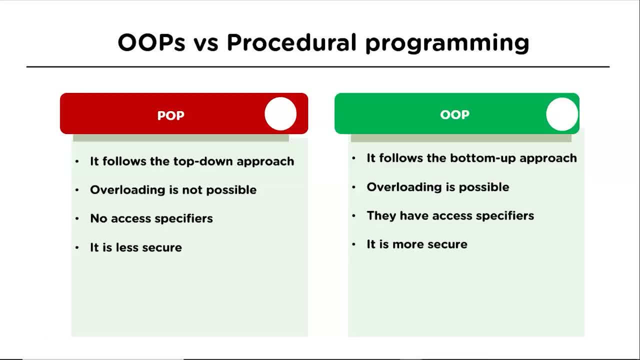 means piecing together smaller tasks to give rise to complex tasks. In procedural programming. overloading is not possible In OOPs. overloading can be done In procedural oriented programming. there are no access specifiers In OOP. they have access specifiers like private protected. 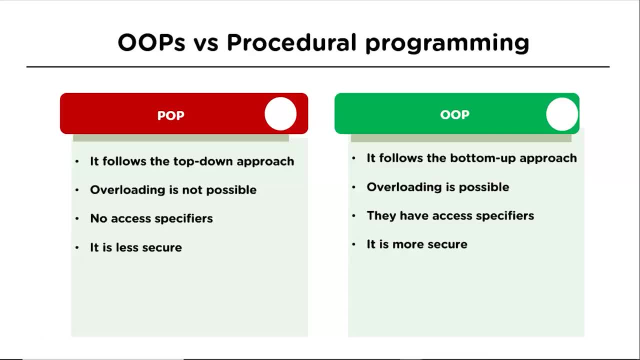 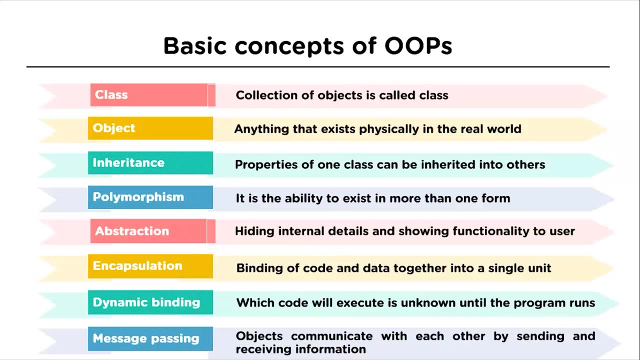 public, Procedural oriented programming is less secure. OOPs is more secure because of the concepts like abstraction and encapsulation, which are used for data hiding. Now let's learn the basic concepts of OOPs. First is class. Class can be defined as collection. 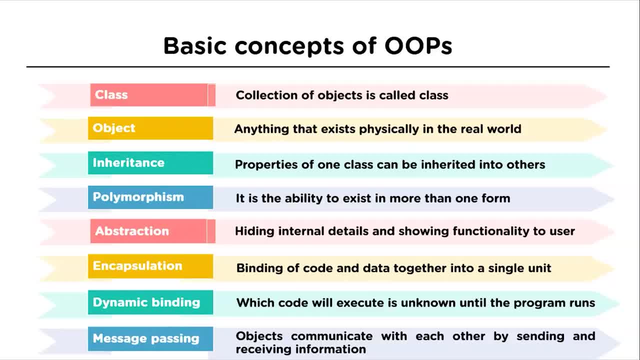 of objects. It is a logical entity. Then there is object. It is defined as an entity that has state and behavior, Or in other words, anything that exists physically in the world is called an object. Inheritance can be defined as when one object acquires properties and behavior from its 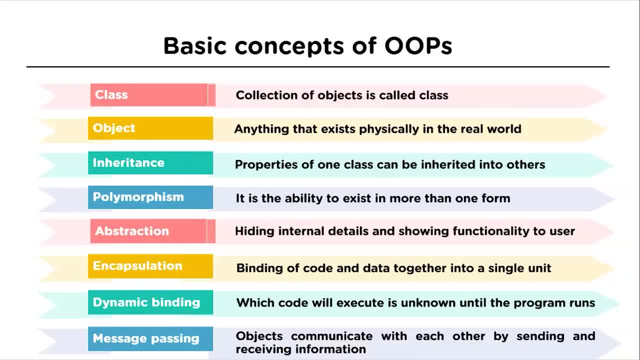 parent class. It provides code usability. Polymorphism is a combination of two words: poly, which means many, and morphs, which means forms. It is basically an ability to exist in more than one form. Next is abstraction. Hiding the internal details and showing the functionality to the user is called abstraction. 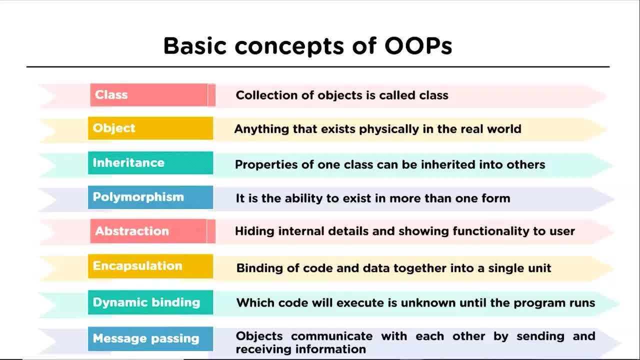 Then encapsulation. Encapsulation is the binding of code and data together into a single unit, Dynamic binding. Dynamic binding is the method called at runtime. that means which code will execute is unknown until the program runs. Then there is message passing. It is basically a communication that exists between the objects. 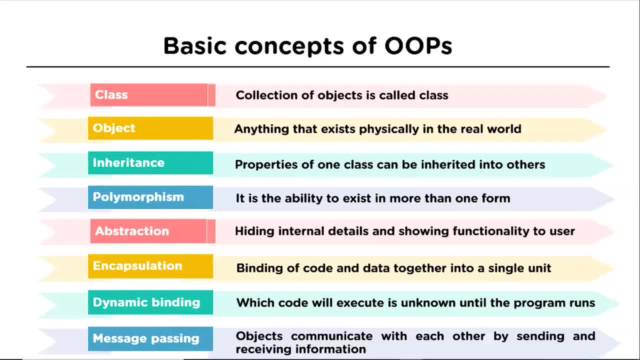 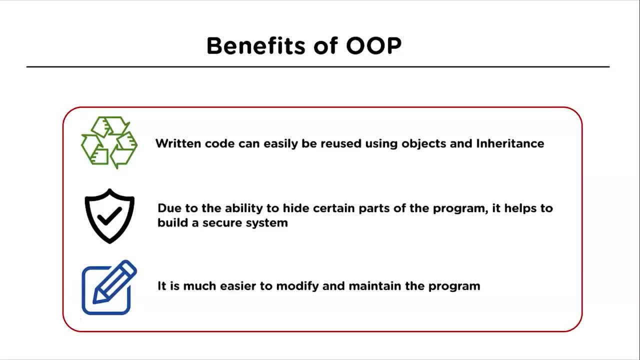 As we have gone through some concepts of OOPs, now let's discuss some benefits of OOPs. In OOPs, code can easily be reused with the help of inheritance and object. We don't need to write the same code over and over. 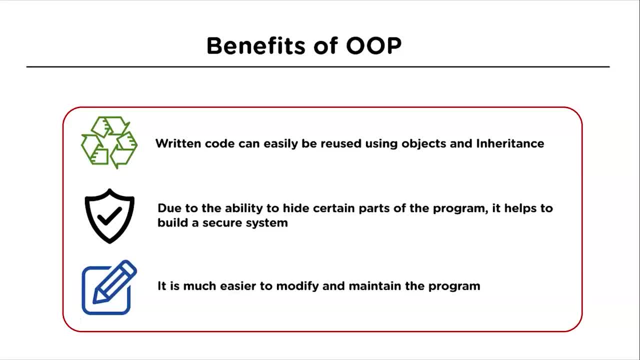 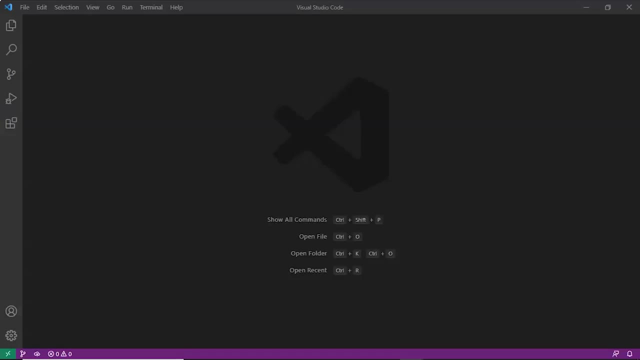 Second is, with the help of abstraction and encapsulation, certain parts of program can be hidden and it helps to make a secure system. Third is maintaining and modification of code. It is easy in object-oriented programming Now to do some examples on concepts of OOPs. let's move on to a code editor, that is, VSCode. 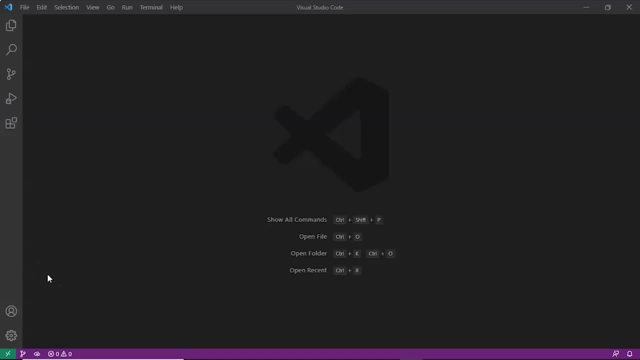 Now, here we will do a program of inheritance in which we will make a parent class and a child class and we will call the attributes using object of child class. So let's get started. First of all, let's name the file. Let's name the file. 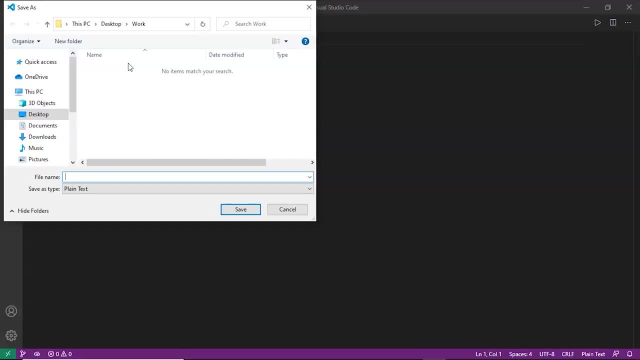 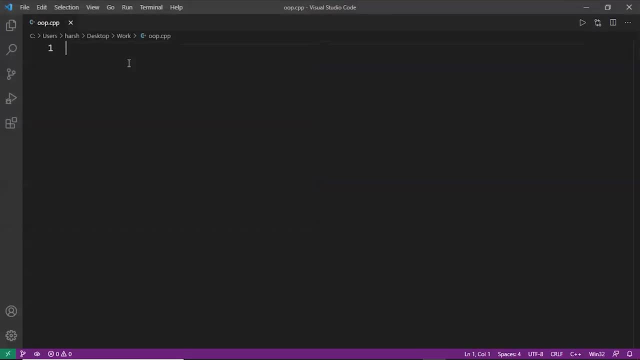 Let's name the file. We will write OOPcpp. We will write OOPcpp. Okay. So first of all, we will add the header files. Hash include Iostream: Now adding namespace standard. Now we will write int main. so we want to create the object of child class. so first of all, 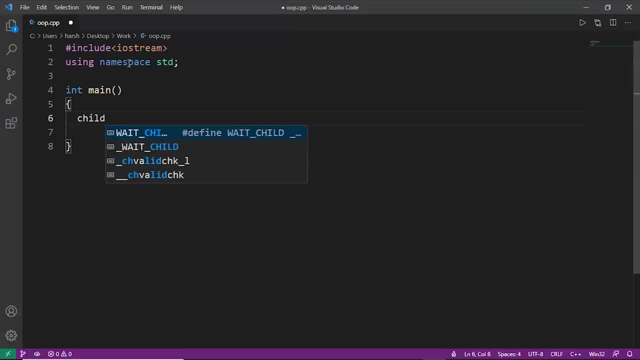 we will write the name of class child, that is, child- let's put C, capital child- and now the name of the object CH. so now we will call the attributes using this object. so we will write, first of all, display it. so we will write chname One, which is the attribute we will. 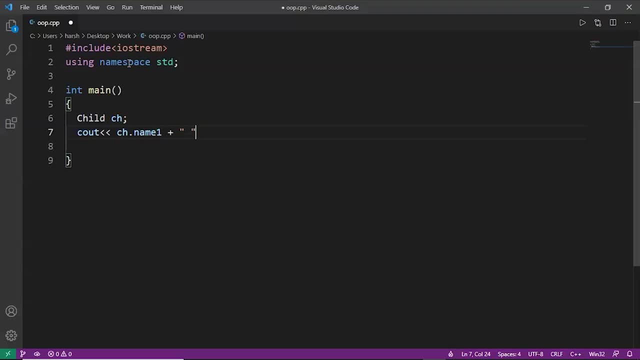 declare it later. Ok, so basically we want to write both the names of both the classes together. so that is why we are doing like this: will write name to name one will be the attribute of the parent class and name two will be the attribute of child class. 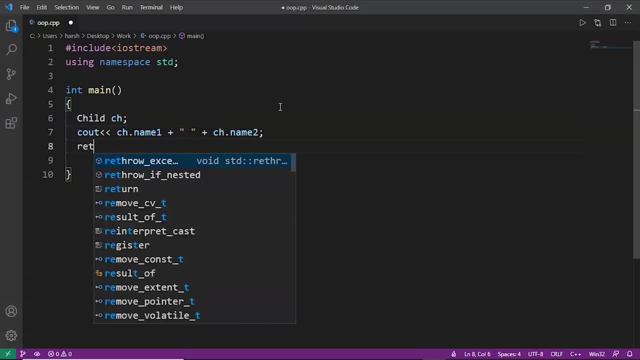 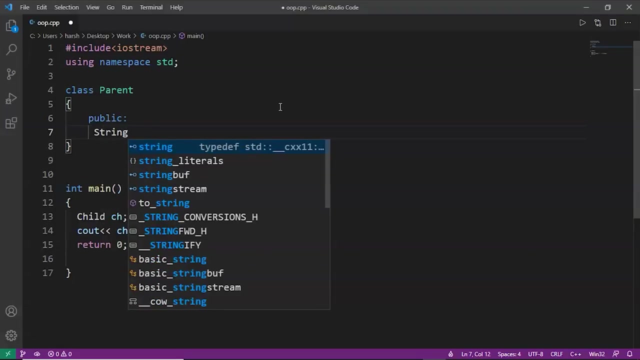 so after that we'll write return zero. now we'll make the parent class and the child class. so first of all let's write class parent will name it as parent. then we'll write public access. specifier string is the data type name one. let's write harley. 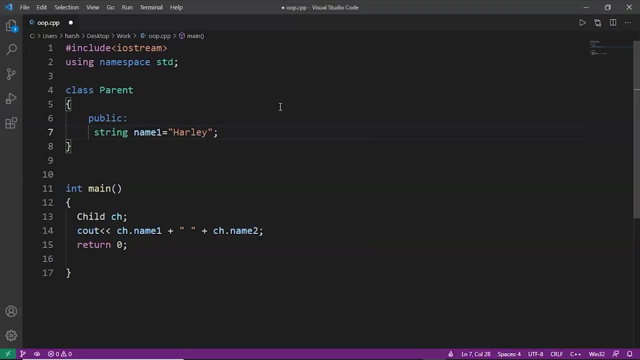 okay, now it is mandatory to write the semicolon at the end of the class. now we'll write the derived class, that is child. we will write the child class. we will write the child class, the colon symbol. then we will write public name of the parent class, that is parent. so 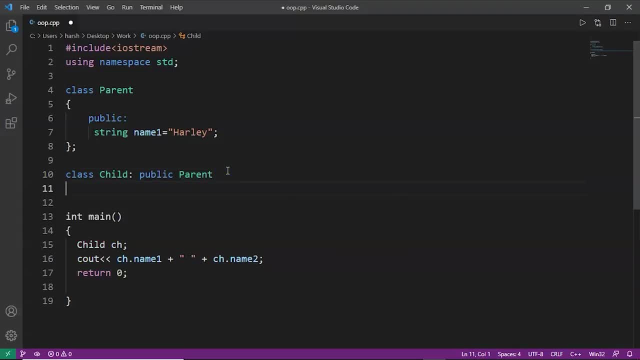 here we are writing: the child class is derived from the parent class. now within the bracket we will write public, then string the datatype name to. we will write Davidson. it's a popular bike brand, Harley Davidson. so now we will write the semicolon over here. now we will. 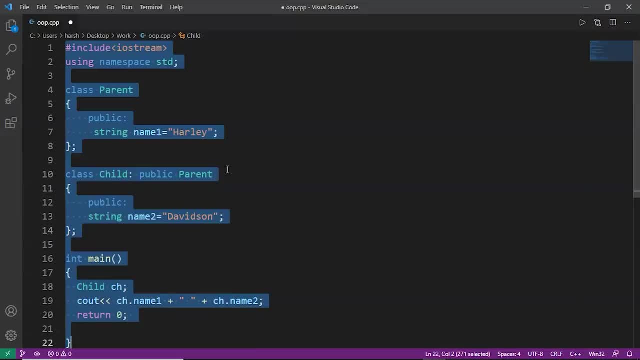 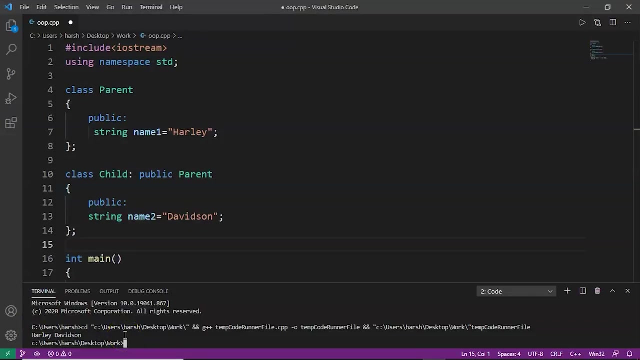 try to run this so as we can see Harley Davidson here, Harley is from the parent class and Davidson is from the child class. so as we can see that we are calling from the object of child class and still we are able to access the attribute of parent class. 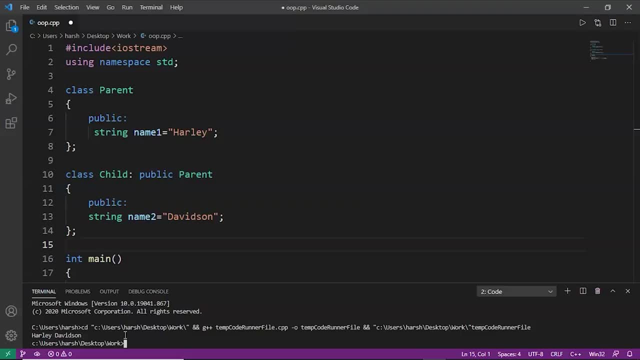 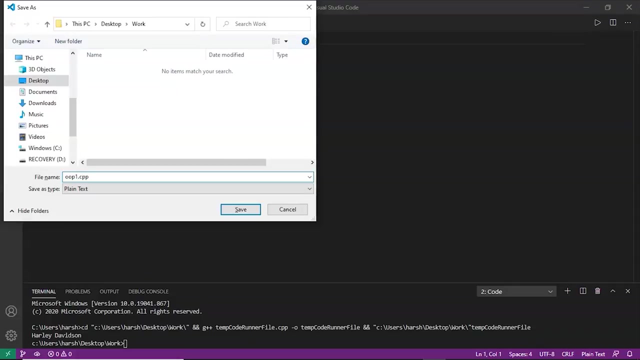 so this shows that the child class inherit attributes or properties from the parent class. now, as we have done one example of inheritance, so now lets do one example of polymorphism. also, lets name it hoop1.cpp. first of all, we will include the header files. so add list, add list. 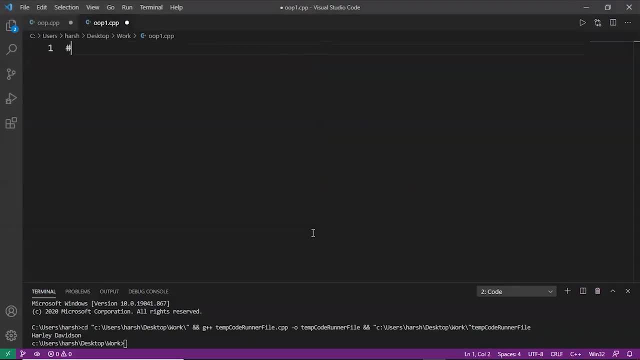 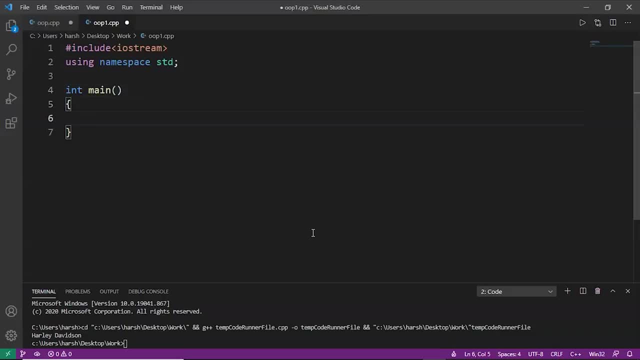 int main. now, here we will do an example of polymorphism, in which we will make a base class and it's derived classes, and inside these classes we will override a function which is common in all of these classes. so let's start. first of all, we'll write the name. 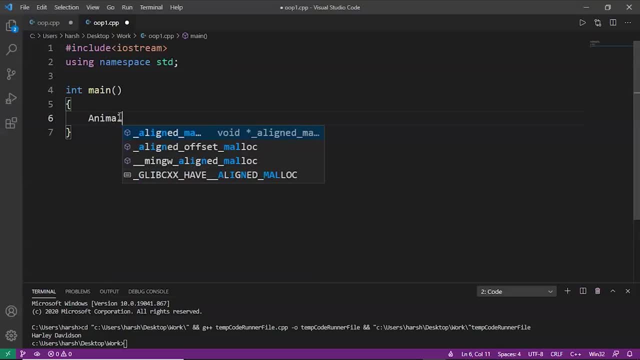 of the parent class or base class animal and we'll make an object a. after that we'll write the name of the child class, Jita, and its object name is C. let's say now another derived class, dolphin, and we'll name the object as D. now, while making 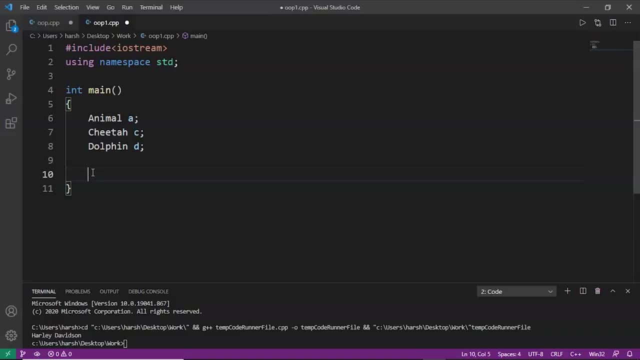 these classes, we'll write a function named speed in all of these classes, inside all of these classes. and now, in order to override that function, we'll call them. so, first of all, we'll call it by the object of animal, that is, a dot speed- now c dot speed. this is the object of Chita class, now D dot speed. 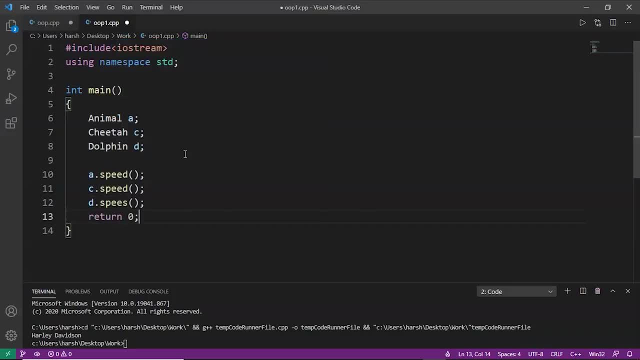 after that we'll write return zero. now let's make these classes first of all. we'll write: First of all, we will make the animal class, that is the base class, animal. Now we will write the access specifier: public. Now we will write the function void, that is the data type: speed. 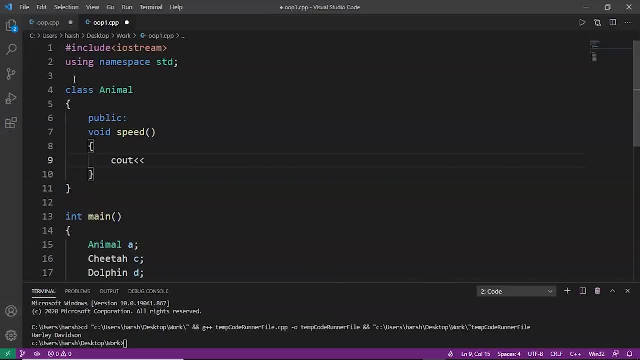 Now we will display a message inside this function. Let's say it displays who is more faster. who is more faster? okay, Now we'll put a semicolon in the end. Now we will make a derived class. that is dolphin. We'll write class. 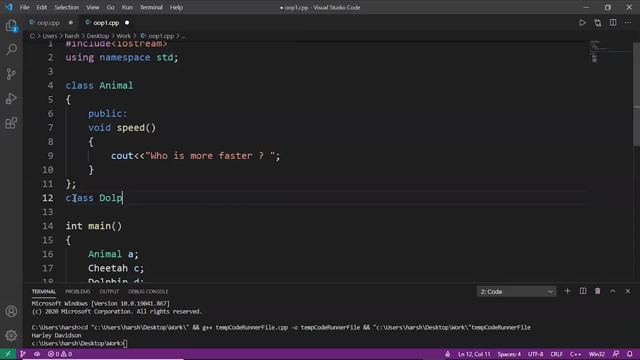 Dolphin, child of animal class. Okay. so now inside this class, we'll write public and we'll make the same function speed. Okay, Okay, Okay, And we'll display a message saying: as this class is of dolphin, So we'll write. I'm faster in water. 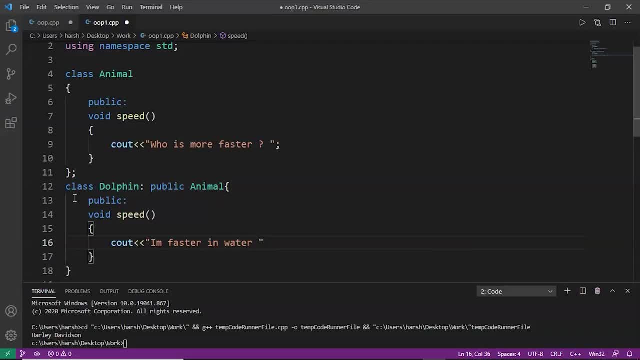 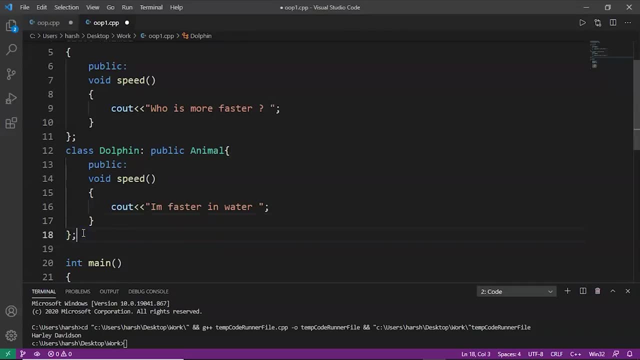 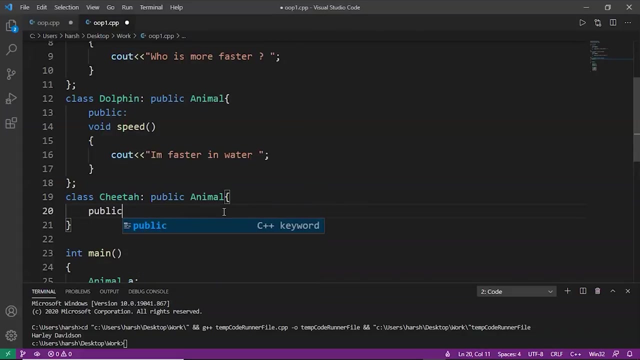 Okay, Okay, Okay, we'll put semicolon. now we'll make another child class class cheetah. okay, C is capital cheetah, public animal. now, here we will write public access specifier, and we'll write the same function, void speed, and over here we'll. 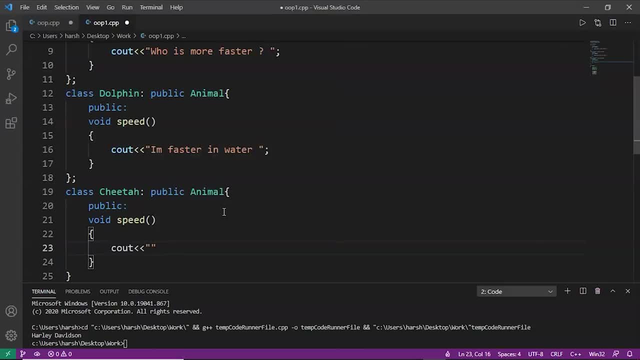 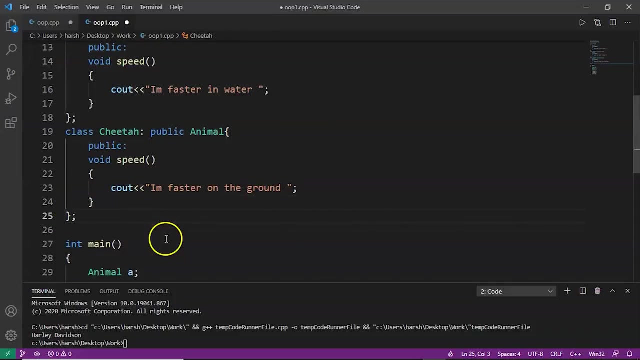 display a message saying that I am faster on the ground. this is null semicolon. so now, as we can see that aspeed is calling this speed function in animal class, cspeed is calling this cheetah function in cheetah class and dspeed is calling the Dolphin speed function in Dolphin class. 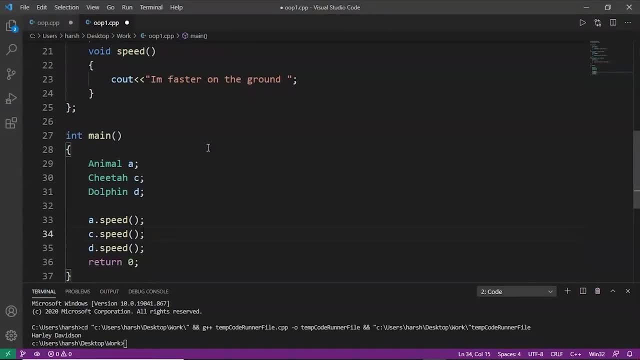 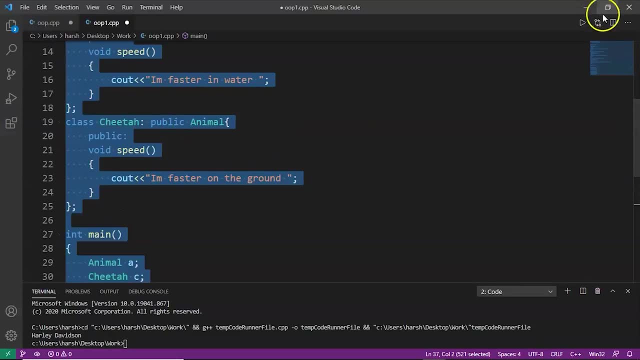 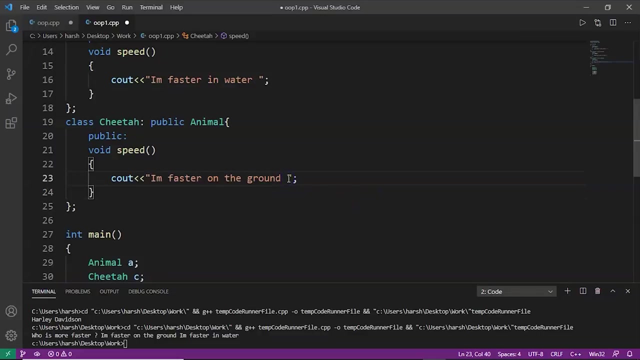 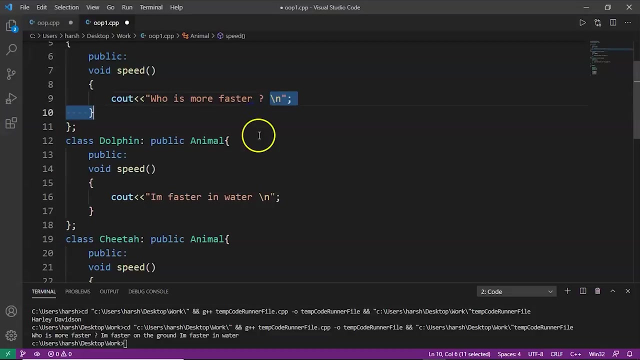 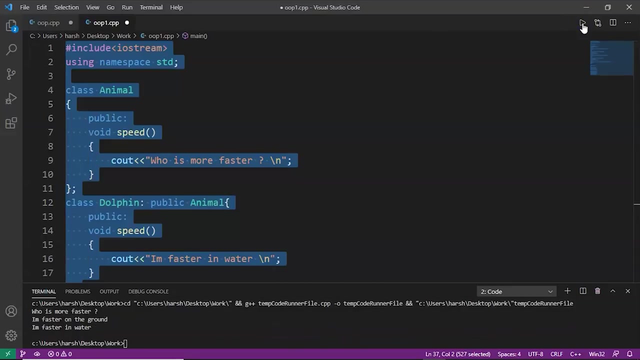 okay, so now let's try to run this. okay, the output is here, but it is not in very good form, so let's put slash n in the end. okay, slash n, slash n. okay, here it is. so first who is faster is displayed, then I'm faster on the ground, then 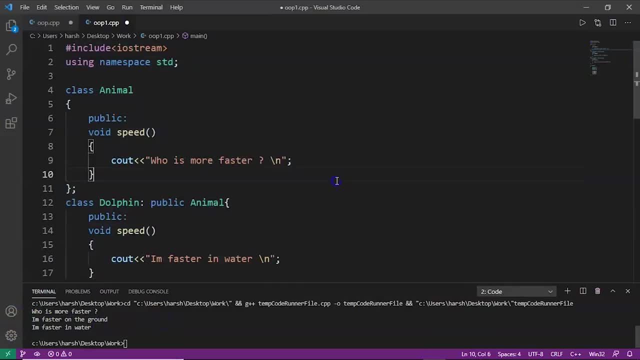 I'm faster in water is displayed. so as we know that first of all we have called the animal class, so that is why who is more faster is displayed. after that we have called the cheetah class, and cheetah says that I'm faster on the. 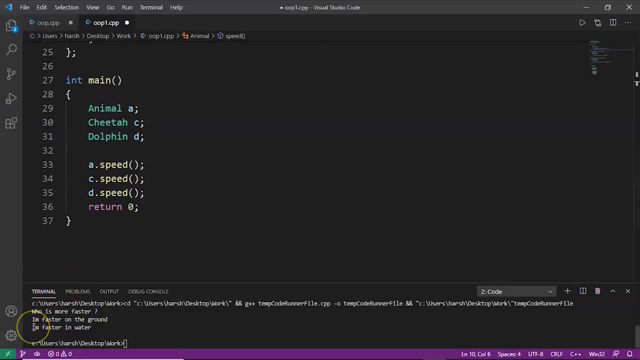 ground, then dolphin class. then dolphin says: I am faster in water. so here we can see that each of the class have its different implementation for the same function that his speed. and this is how polymorphiestm allows us to do a single action in varity of. 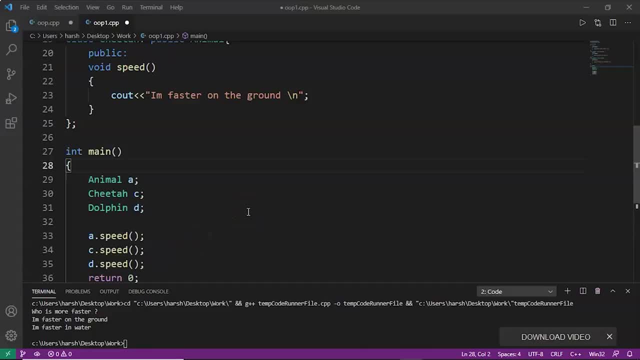 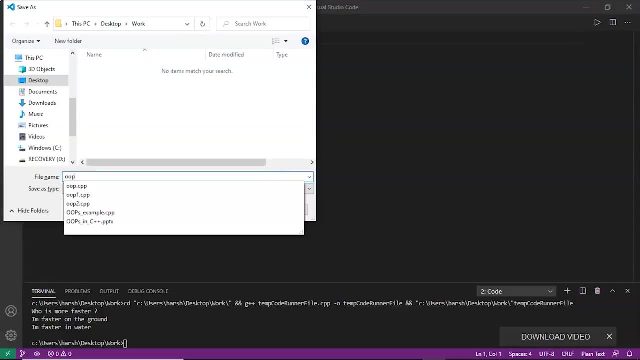 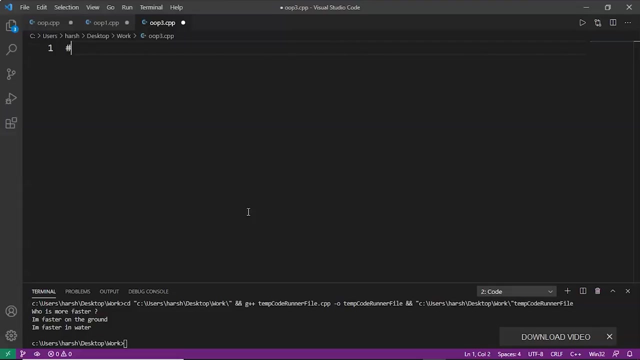 ways. okay, now let's do one example of abstraction. let's name it: has whoop threecpp, first of all, will include the header files. will write hash. include is przed stream. Now we'll write the namespace standard using namespace std. Now, as we know, abstraction. 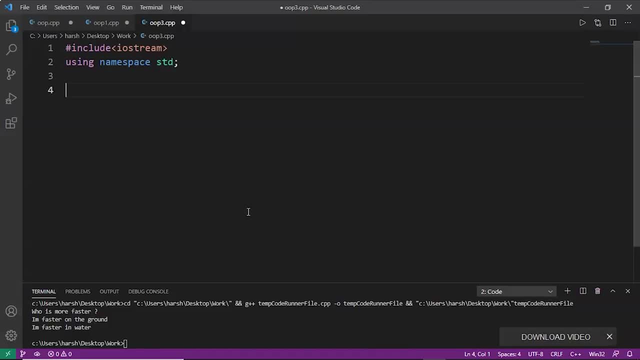 helps in data hiding. So in this program we will make a variable named coupon as private And with the help of set coupon function we will try to assign some value to the coupon variable And after that we will display it. So let's start. First of all, we'll write. 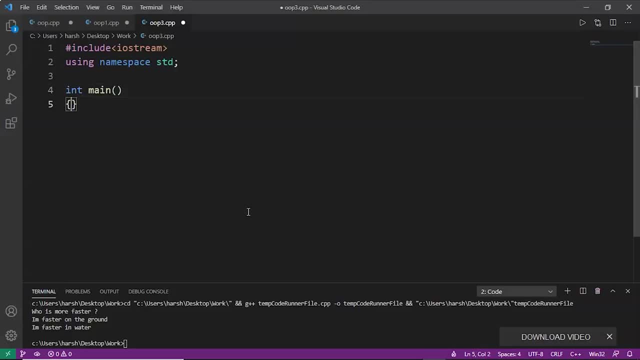 int main. Now we'll write the name of the class, that is, trade fair, trade fair- And now the name of the object: T. Now, with the help of this object, we will call a function named set coupon. I would say coupons, And we'll pass 50 as an argument to this function. Now we'll display: 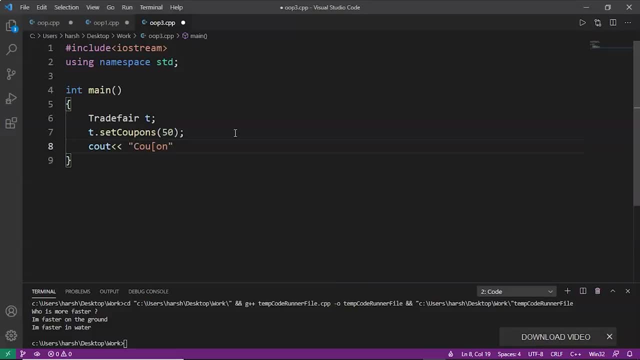 a message coupon, And after that we will call get coupon method in order to display the number of coupons. So we'll write T dot, get coupons and brackets. Then after that we'll write return zero. Now let's make the class and the functions. 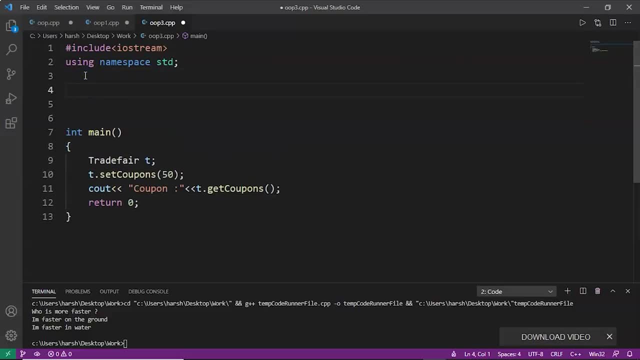 So let's start. First of all, we'll write class trade fair. Now we'll write an access specifier private And I private. Now we will declare a variable coupon. Now we will declare a variable coupon And, as I've already told you, we will make this variable as private. So that is why we 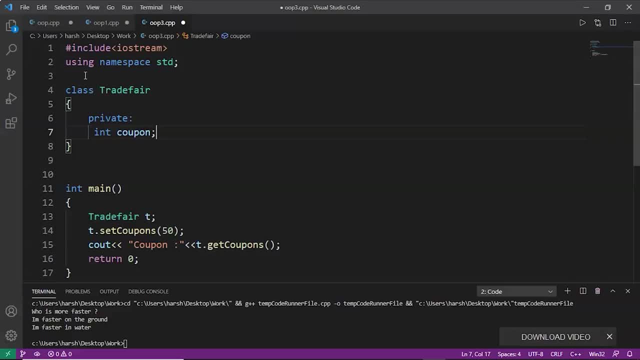 have used this access specifier as private. Now, after that, we will write public access specifier to write a function that is set coupons Set, coupons Set, coupons Set. Now we will write a value of 50. And the parameter is C, as we know that we have passed 50 to this parameter, So now we 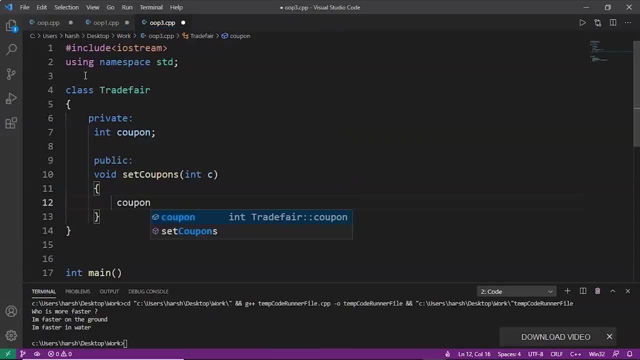 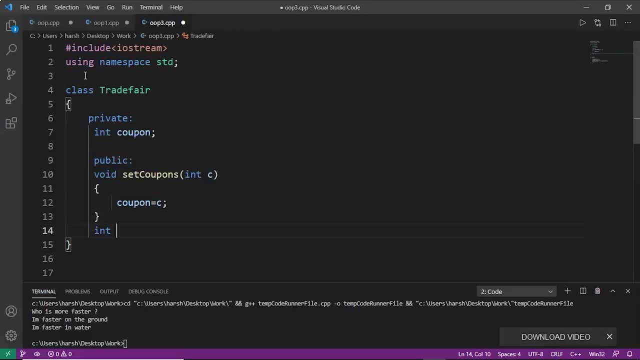 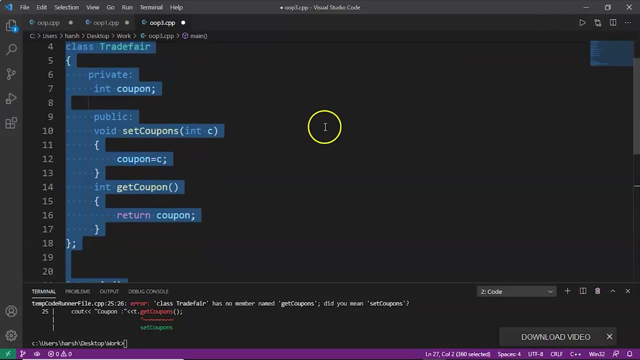 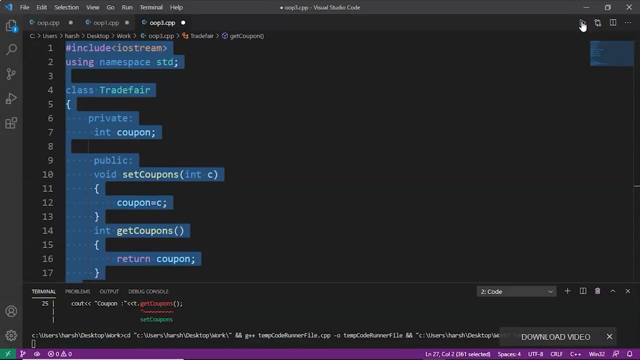 because it is returning something. so we'll write int- get coupon and we will return variable coupon. now, as the class ends, we will write semicolon. now let's try to run this code. there is some error, you okay, we haven't right s over here. now let's again try to run it. 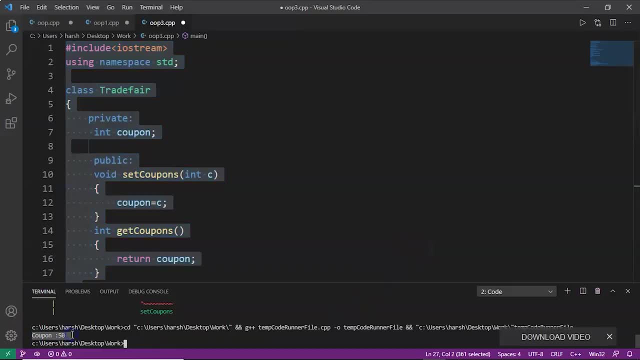 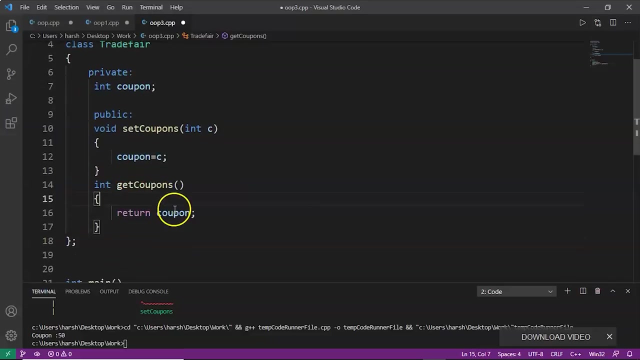 coupon 50, as I've told you. so here we have assigned 52, this function, and the variable C is assigning 52, the variable coupon. now, after that, we have used get coupon function to return the value of coupon and that is why it is getting displayed over here. so we got our answer, that is, coupon 50, and, as you, 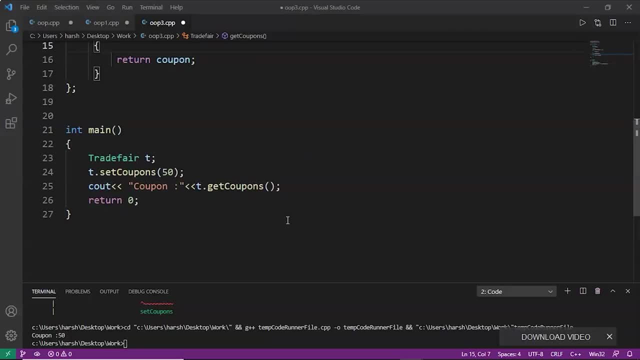 can see that in this example we are not allowed to access the variable coupon, but still, somehow we have managed to do that with the help of some function. and we are going to right: select this promised variablek цe PowerPoint and we've got our answer. 50. and, as you can see that in this example we were not allowed to access the variable coupon, but still, somehow we have managed to do that with the help of some function. bye, bye.